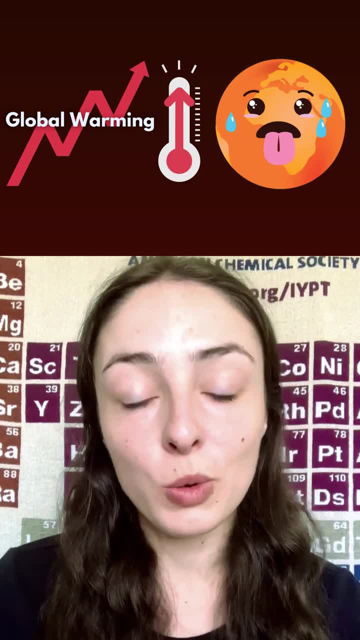 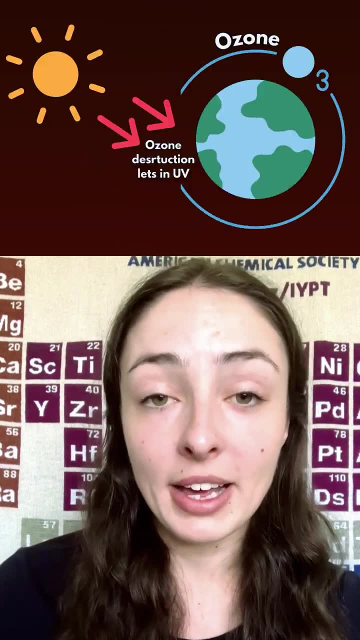 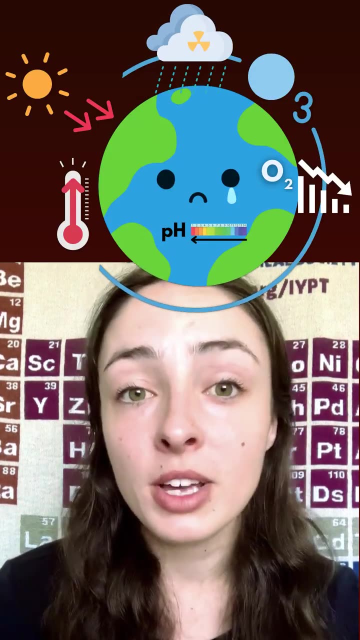 among the organisms. They did, however, cause rapid global warming ocean anoxia or oxygen depletion, ocean acidification, ozone destruction and increased UV radiation and acid rain. Together, these rapid climate changes created the perfect storm of extinctions across both. 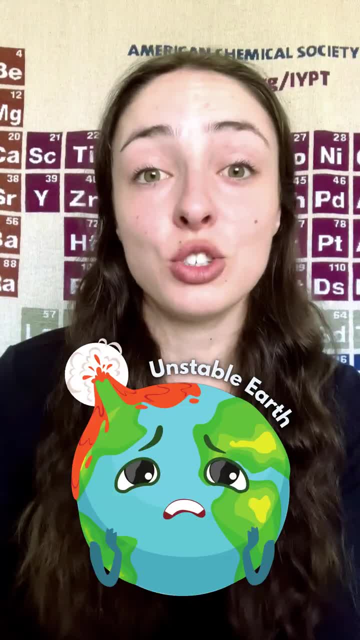 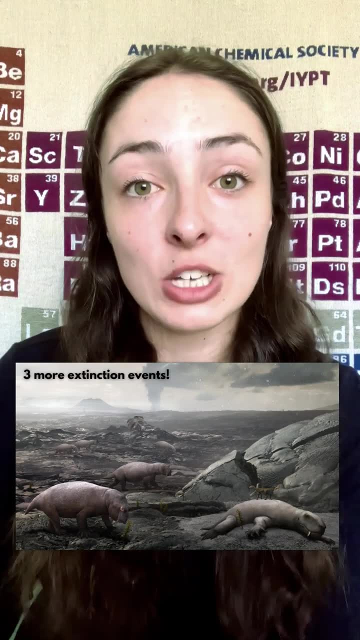 the marine and terrestrial realms. In fact, Earth was left so unstable after this event that three more consecutive mass extinctions occurred right after this event in the early Mesozoic era. But this wasn't bad news for all life. This actually virtually emptied all terrestrial niches, for dinosaurs to take over, which is why they then ruled the next 200 million years. 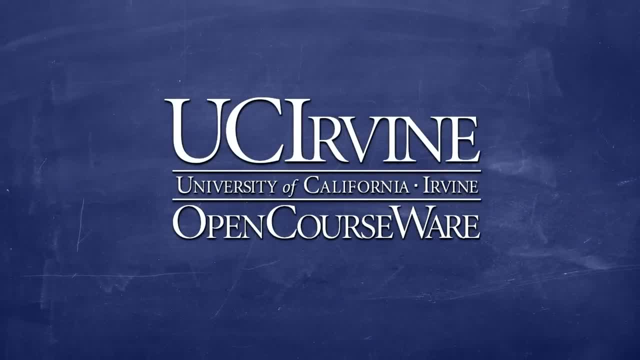 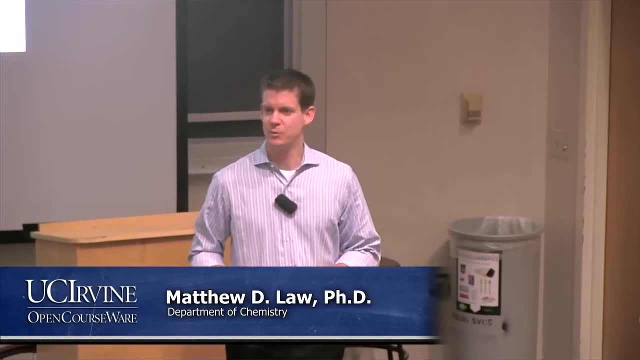 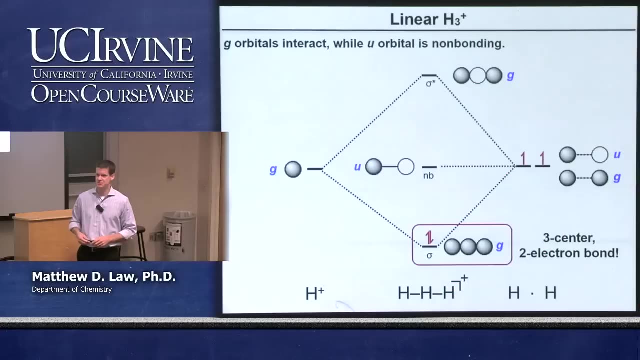 Okay, so last time we were just beginning to build more complicated molecules. Our first three atom molecular orbital example is shown here. This is where we ended, Where we did the molecular orbital diagram for H3+, And remember, what we're doing in these cases is we're going to break the molecules up into group orbitals. 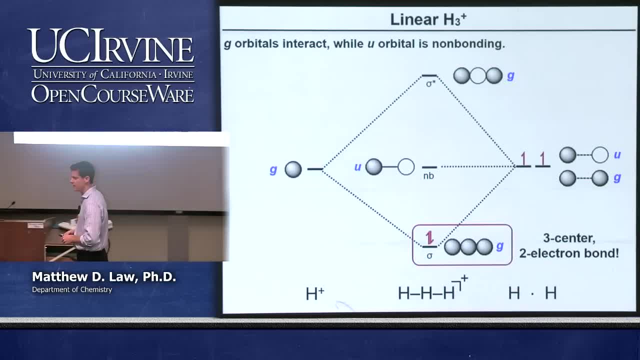 and then a central atom, a center atom, And what we did here is we used the two outer hydrogens as our set of group orbitals, right 1s orbitals from each of those outer hydrogens And the center hydrogen is the central atom. 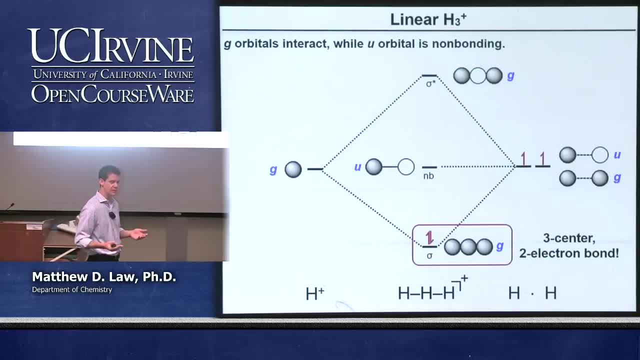 And we found what the symmetries are going to be just by inspection of these group orbitals in the center atom orbital And then we mixed them according to their symmetry matching And we came up with this picture where we have either even under inversion or odd under inversion kinds of symmetry.